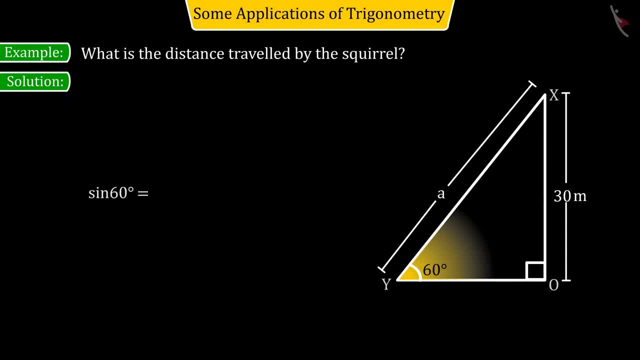 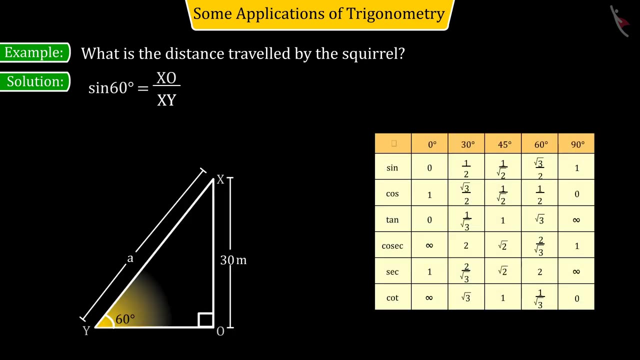 Here from the obtained figure. here from the obtained figure, we get the ratio of the side opposite to theta angle and the hypotenuse, giving us the sine 60 degrees, equal to XO divided by XY. In the left side, there is sine 60 degree whose value is equal to the square root of 3 by 2.. 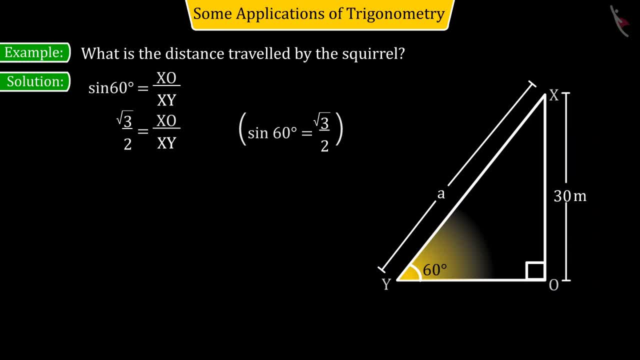